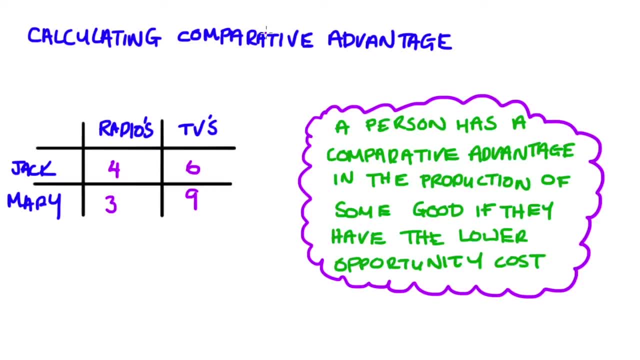 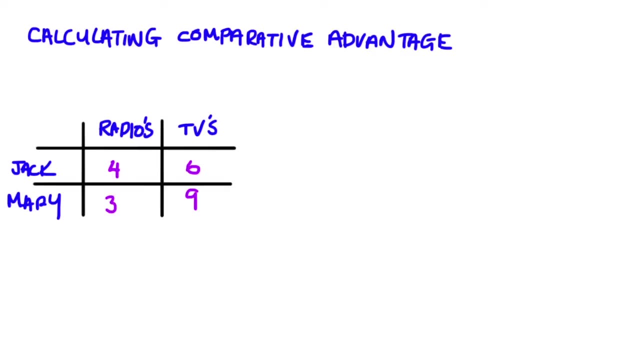 has a country. a country has to give up in the production of another good. So we're going to think about how many radios that Jack has to give up if he makes a TV, or Mary how many TVs she has to give up if she makes a radio, etc. Because it's the case that the production possibilities table. 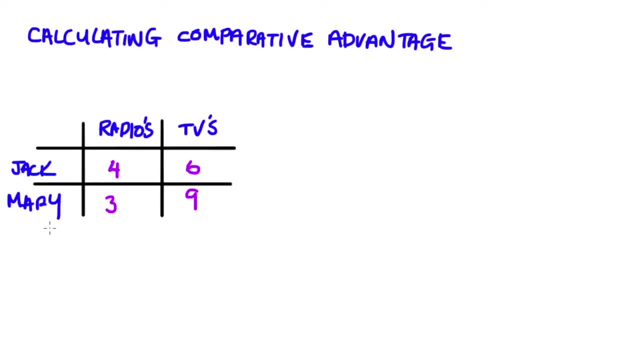 that I have here represent production possibilities. the table really clearly outlines at least a type of opportunity cost. Basically, if Jack spends all his time making radios, he can make four, but he spends no time making TVs so he gives up six TVs. So Jack's opportunity cost of making 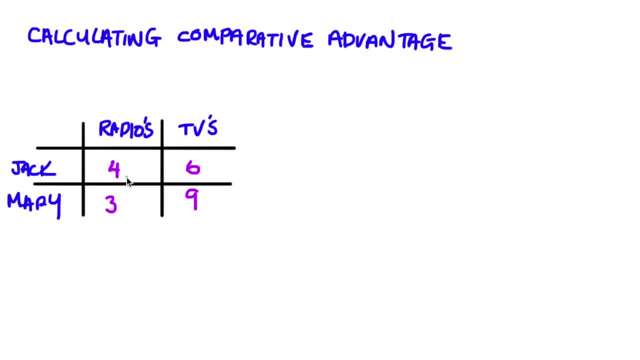 four radios is six TVs. Likewise, if we wanted to understand Jack's opportunity cost of making six TVs, well, if he made six TVs then he didn't have any time to make radios, so he would be giving up four radios. And again, Mary's figures can be interpreted the same way. The 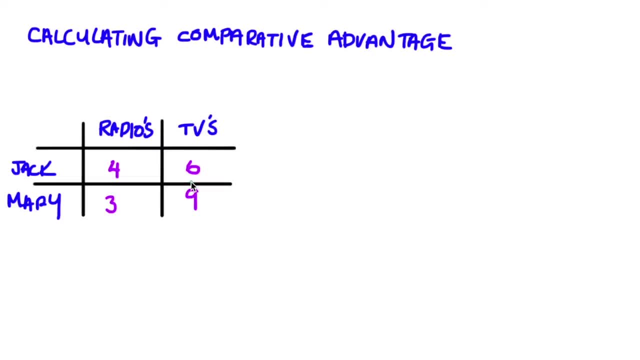 important thing here with comparative advantage is that to assess who has the lower opportunity cost, we need our statements of opportunity cost to be in terms of the same number of the production of each good. So my strategy for working out these sorts of questions is just to modify the numbers. 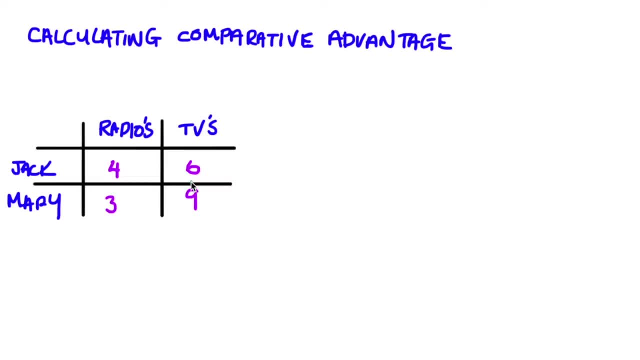 in the table in a systematic way to get our statements of opportunity cost in terms of just one of the type of good. So let's think about radios first and we'll think about Jack. Jack gives up six TVs if he makes four radios, but we want it just in terms of one radio. so what do? 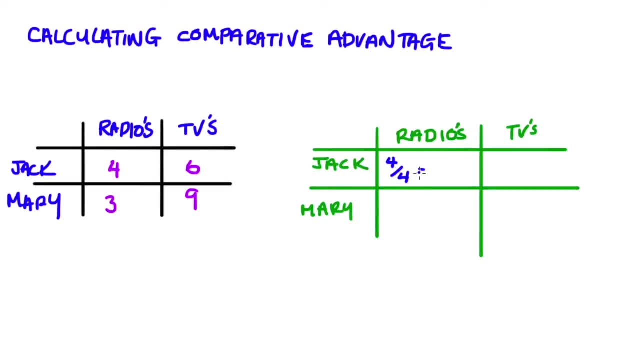 we need to do to four to make it into one. Well, we divide by four, we divide it by itself, but to keep the ratio we have to divide the number of TVs by four as well. so we get six over four, which is equal to three over two, which is one and a half. So if Jack makes one radio, he gives up one and a. 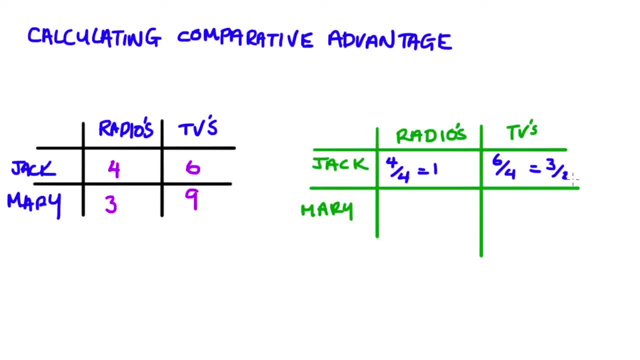 half TVs. We can do the same thing for Mary. so if Mary makes three radios, she's going to have three radios. she gives up nine TVs. but we don't want the opportunity cost in terms of one, in terms of three radios, we want it in terms of one radio. So what do we need to do to three to make it into?